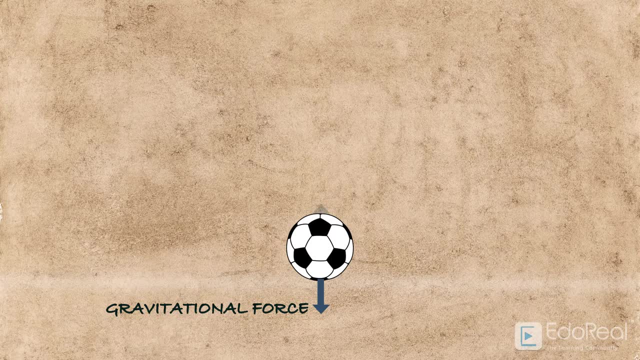 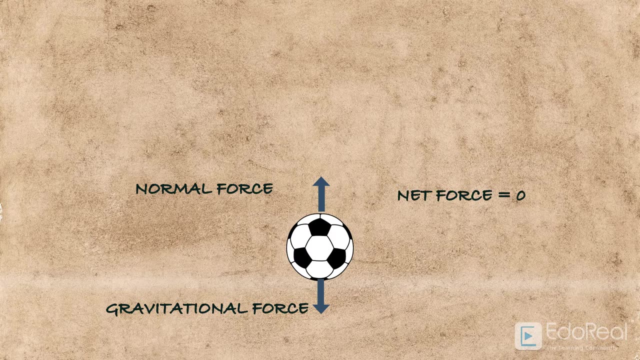 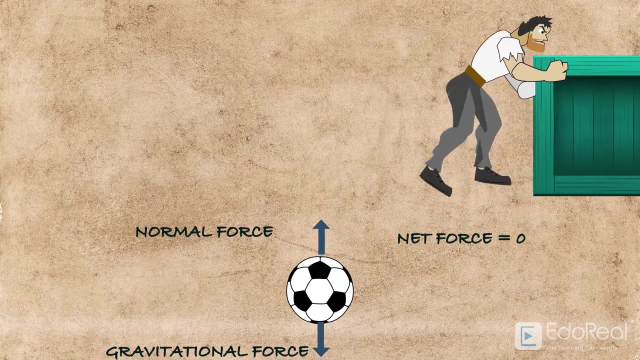 And ground does, applying equal force exactly in the opposite direction, called as a normal force. As these two forces are balanced, the net force acting on the ball is zero, So the position of an object doesn't change. Hence just pushing or pulling is not the only kind of force. 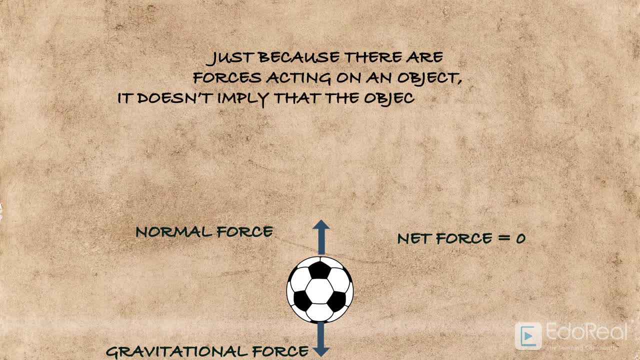 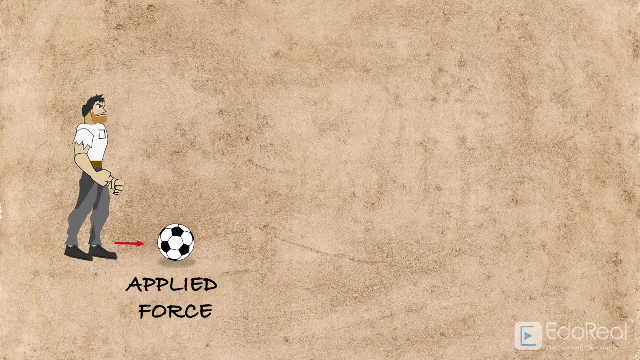 And just because there are forces acting on the ball, it doesn't imply that the object is in motion. There should be some net force for the object to move. If a person kicks the ball, the position of the ball changes due to applied force acting on it. 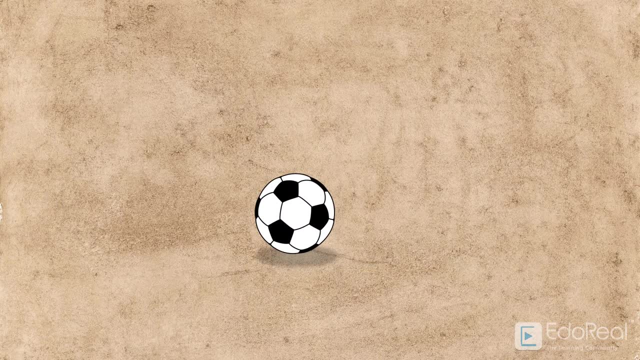 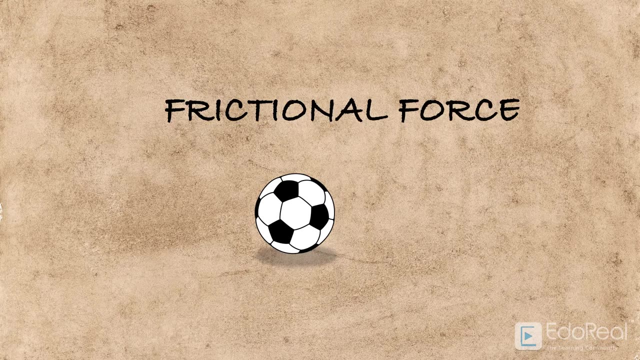 After covering some distance, the ball stops If there is no force from other side. how did it stop? Was there a force which stopped it? Yes, it was frictional force that stopped the ball, If you consider a frictionless floor with no air resistance. 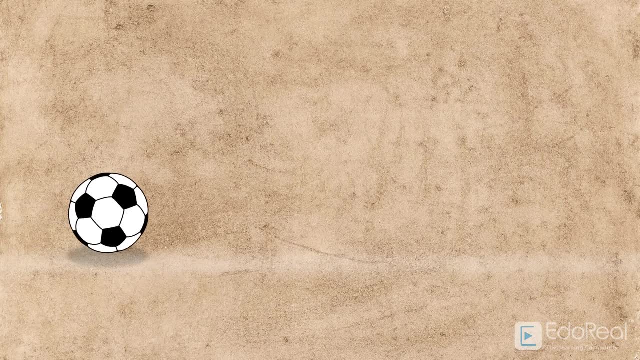 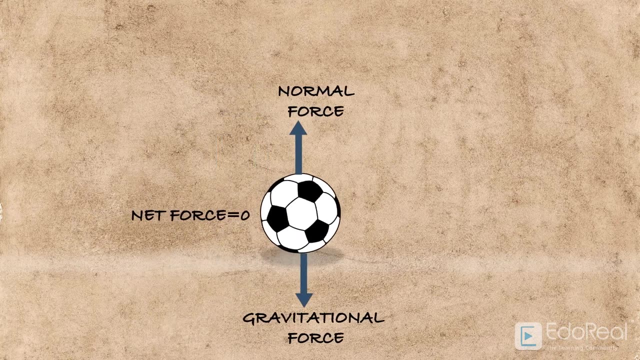 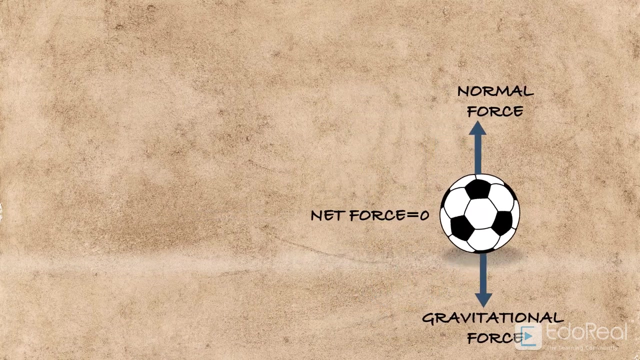 then, for a body moving with constant velocity, the forces acting on it are gravitational force and normal force, but the net force on the body is zero. Now, will the ball ever stop moving? No, it will continue with the same velocity unless there is other external force acting on it. 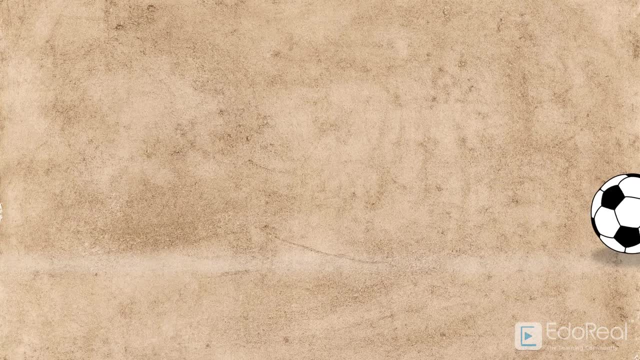 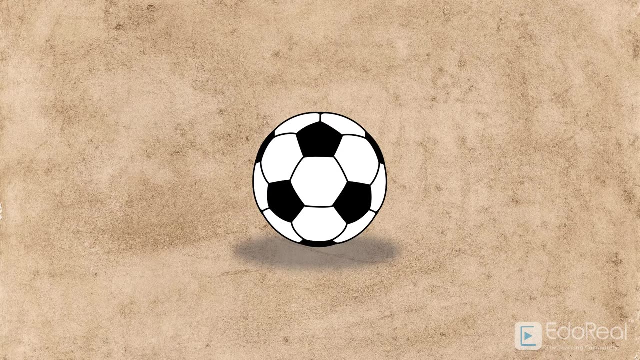 But we assume that if the body is moving then there is some net force acting on it, which is not true. Hence we understood that if the body is stationary, don't think there is no force on it, And if the body is moving with uniform velocity. 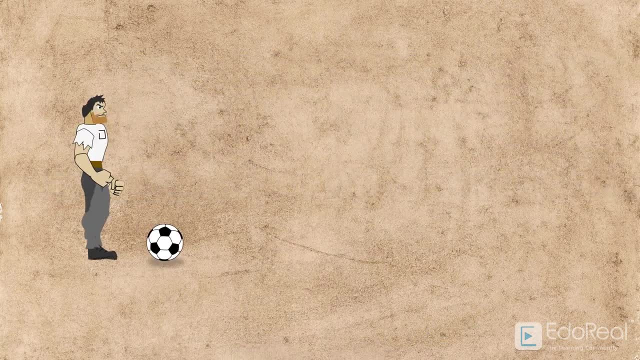 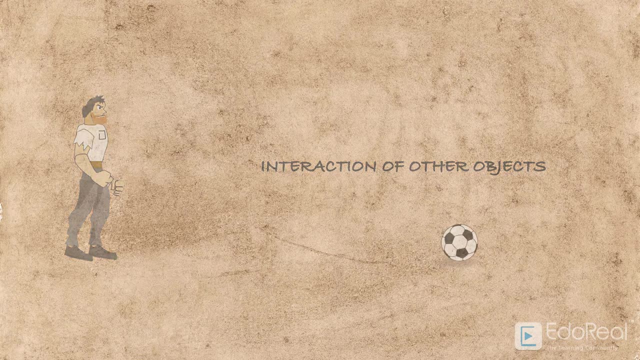 don't think there is some net force acting on it, So force can be explained as a push or pull upon an object resulting from its interaction with another object. If we place a box on a surface which is slant, 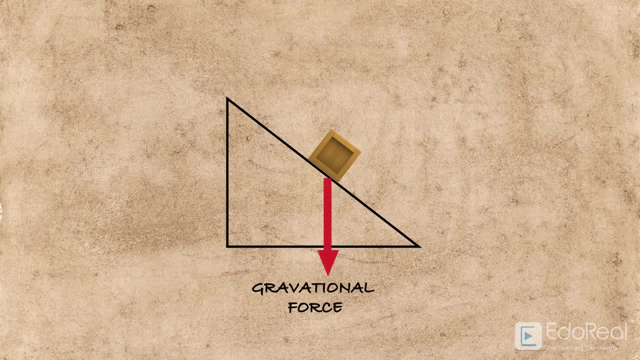 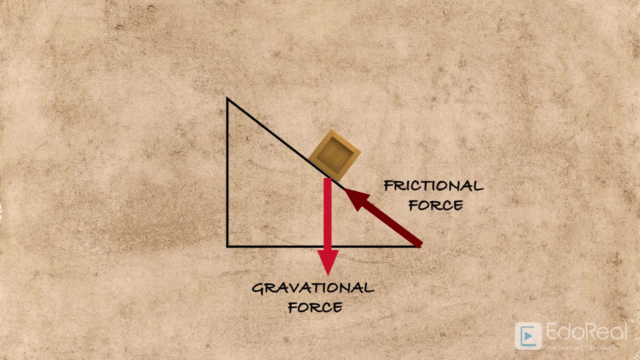 two forces act on the box. one is gravitational force that pulls the box down, and the other is frictional force that acts against the pull. Here, frictional force is a force which is a contact force, whereas gravitational force is without contact. 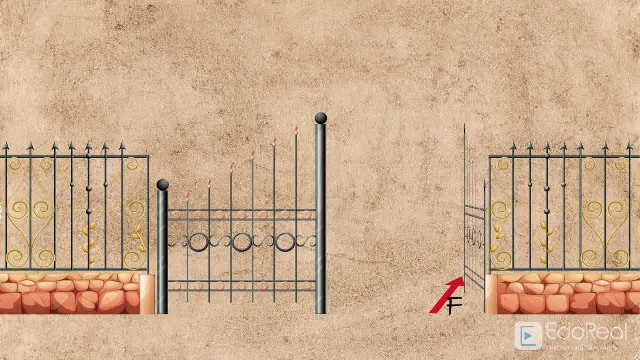 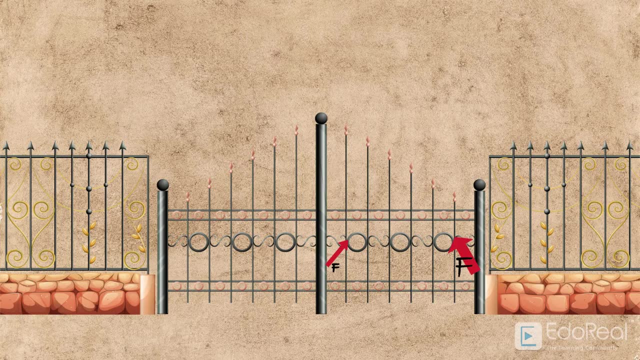 For closing or opening a gate, we need to apply force as per the requirement. that tells the direction And, based on the point of application, the magnitude required will change. Force is characterized by its magnitude, direction and point of application. 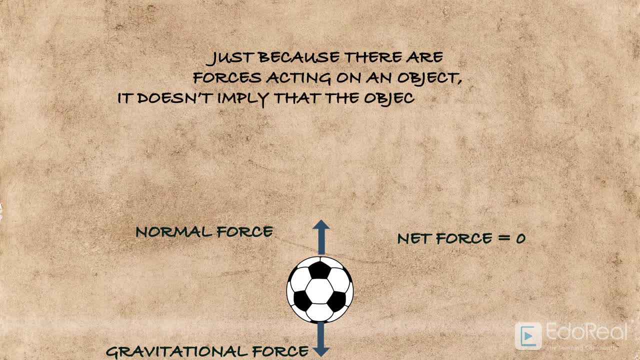 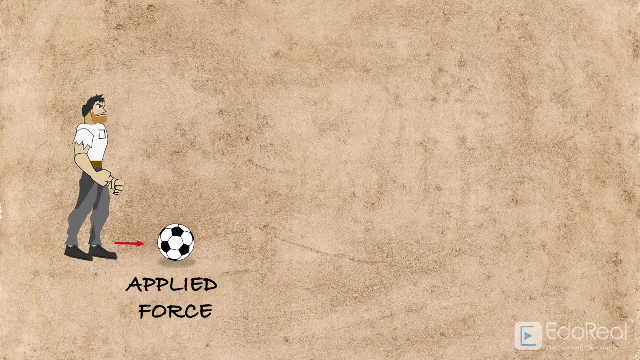 And just because there are forces acting on the ball, it doesn't imply that the object is in motion. There should be some net force for the object to move. If a person kicks the ball, the position of the ball changes due to applied force acting on it. 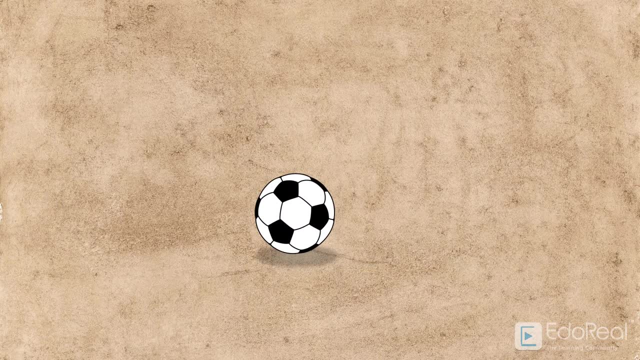 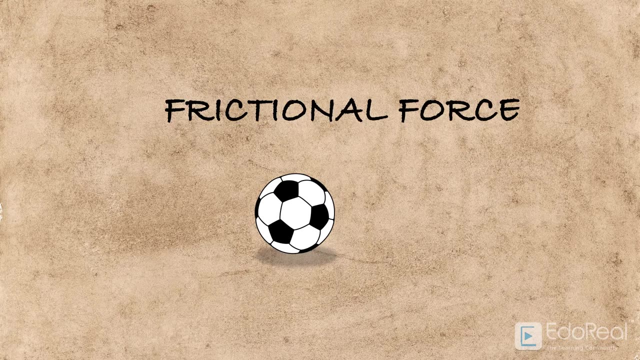 After covering some distance, the ball stops If there is no force from other side. how did it stop? Was there a force which stopped it? Yes, it was frictional force that stopped the ball, If you consider a frictionless floor with no air resistance. 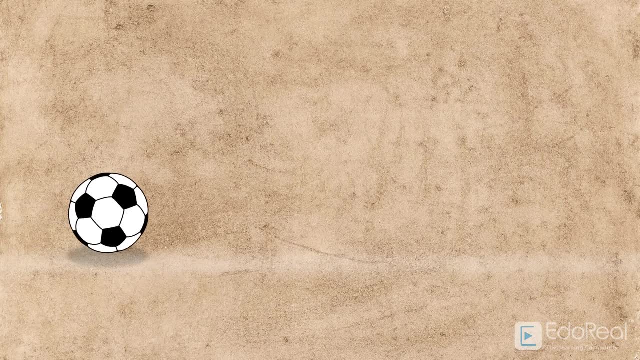 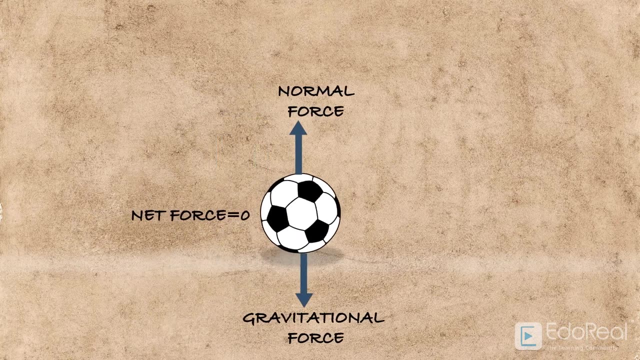 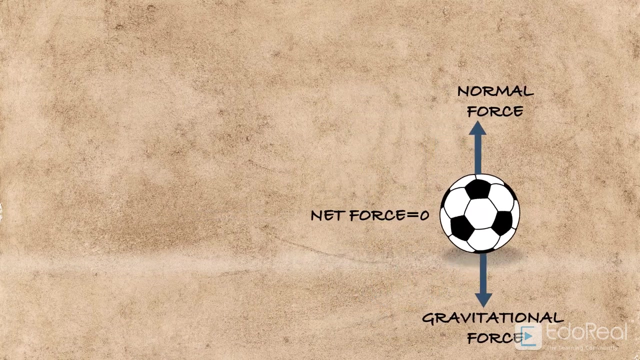 then, for a body moving with constant velocity, the forces acting on it are gravitational force and normal force, but the net force on the body is zero. Now, will the ball ever stop moving? No, it will continue with the same velocity unless there is other external force acting on it. 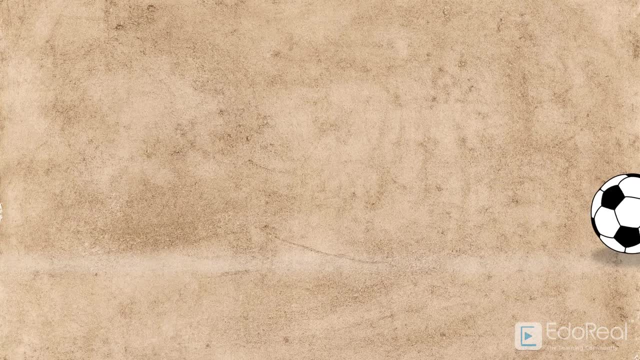 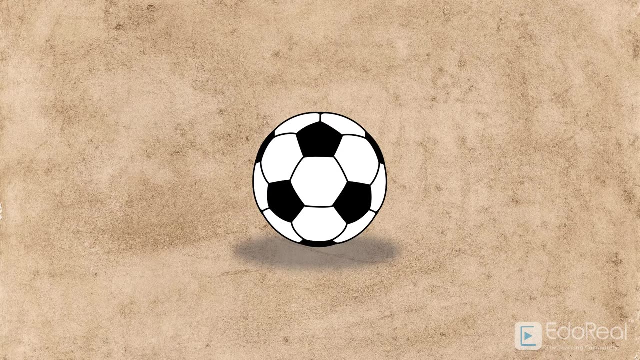 But we assume that if the body is moving then there is some net force acting on it, which is not true. Hence we understood that if the body is stationary, don't think there is no force on it, And if the body is moving with uniform velocity. 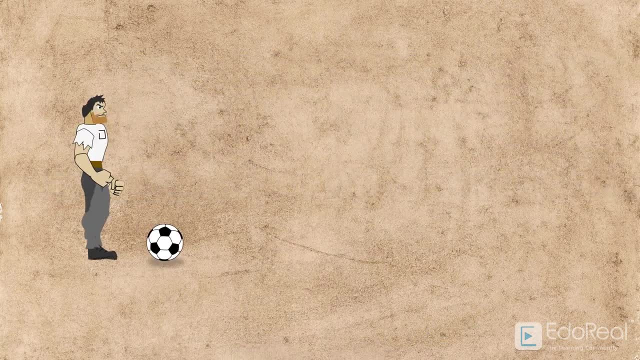 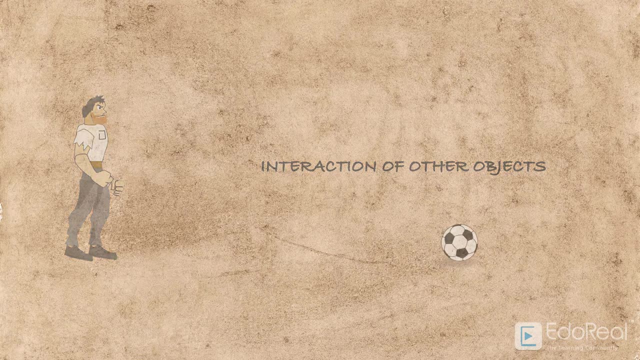 don't think there is some net force acting on it, So force can be explained as a push or pull upon an object resulting from its interaction with another object. If we place a box on a surface which is slant, 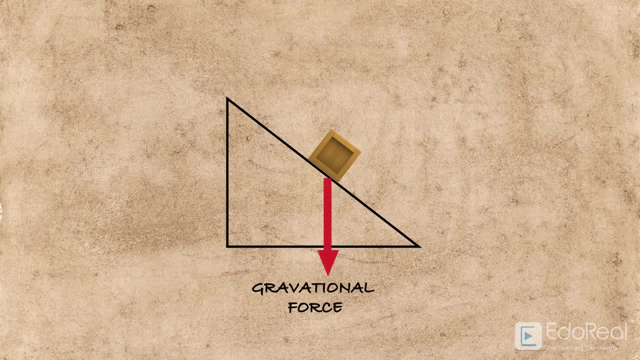 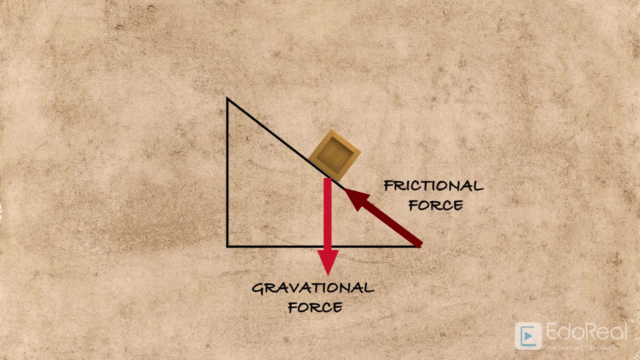 two forces act on the box. one is gravitational force that pulls the box down, and the other is frictional force that acts against the pull. Here, frictional force is a force which is a contact force, whereas gravitational force is without contact. 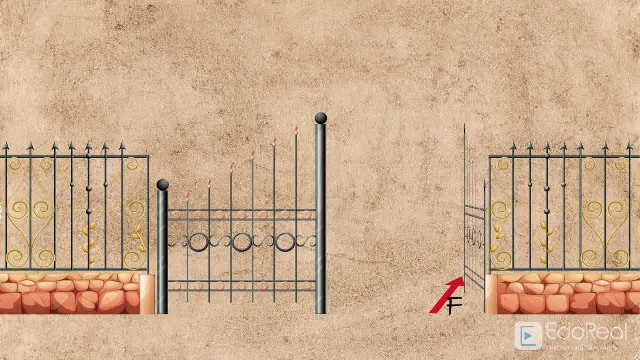 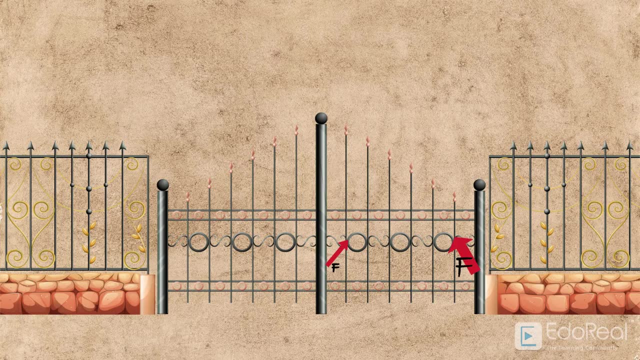 For closing or opening a gate, we need to apply force as per the requirement. that tells the direction And, based on the point of application, the magnitude required will change. Force is characterized by its magnitude, direction and point of application. 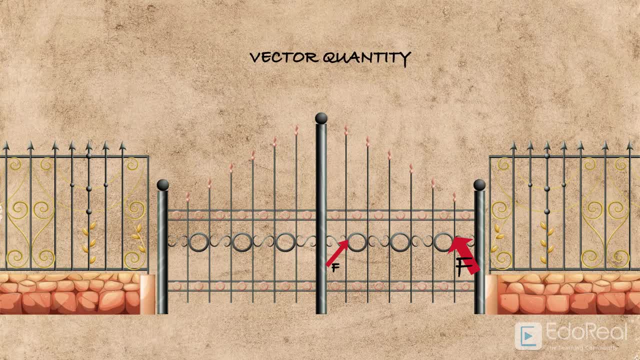 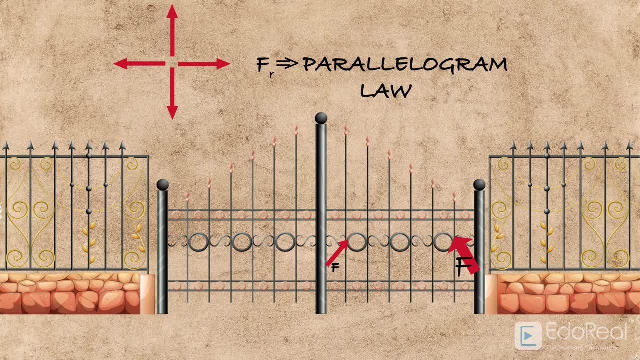 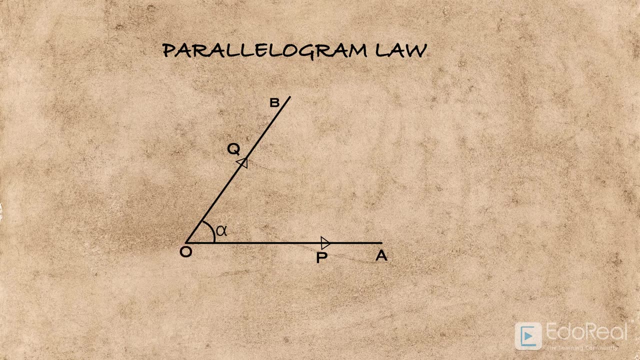 As the force is having direction, it is a vector quantity. If the forces are pointed in different directions, to get the resultant force we use the parallelogram law of vector addition. Let us consider two forces, P and Q, acting on a particle O.